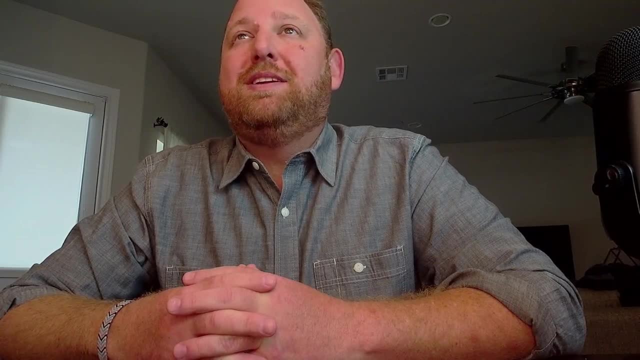 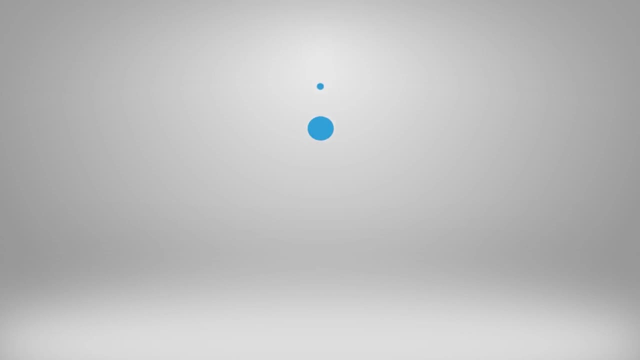 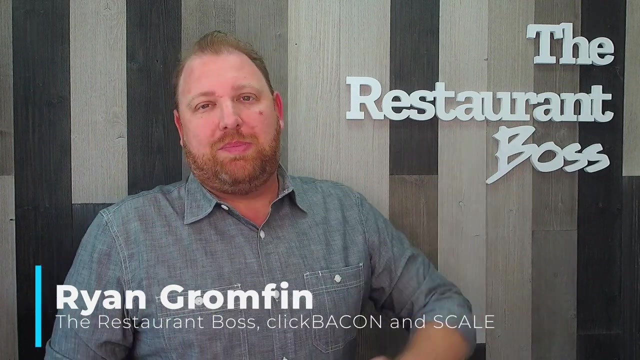 Yeah, this is awesome. You can totally count on me. Great, Do you have any questions? Just one: What's food cost? Hey everybody, Ryan Gromfin here. author, speaker, chef, restaurateur, founder of TheRestaurantBosscom. 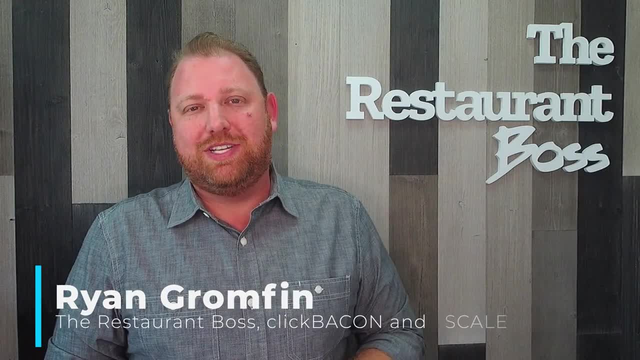 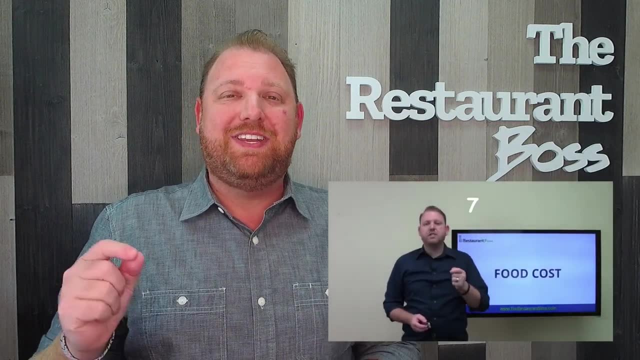 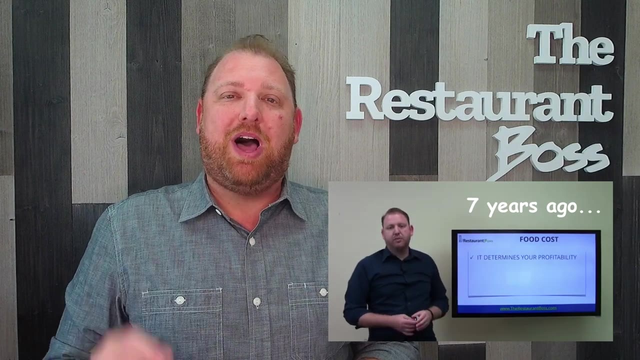 as well as ClickBacon and ScaleMyRestaurantcom. I'm so excited to be making this video. We're basically remaking a video from over seven years ago, One of the first videos I ever put up on YouTube And, to this date, it's one of my most popular. 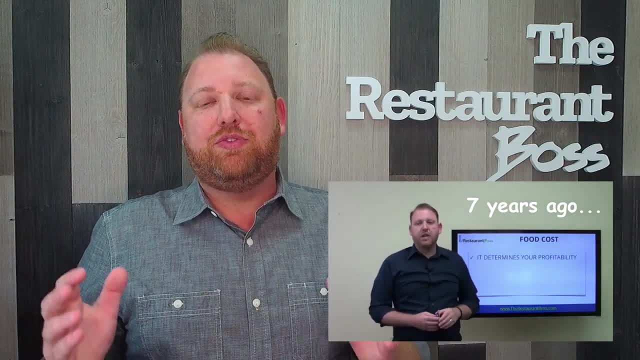 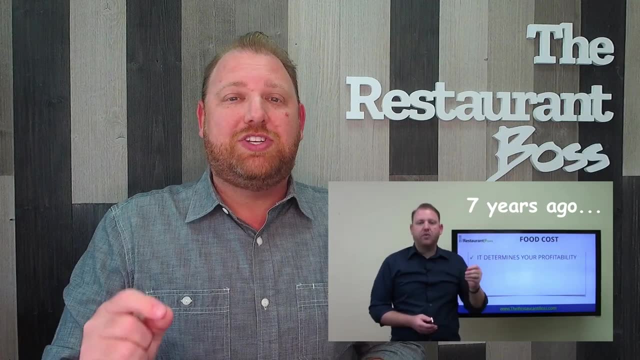 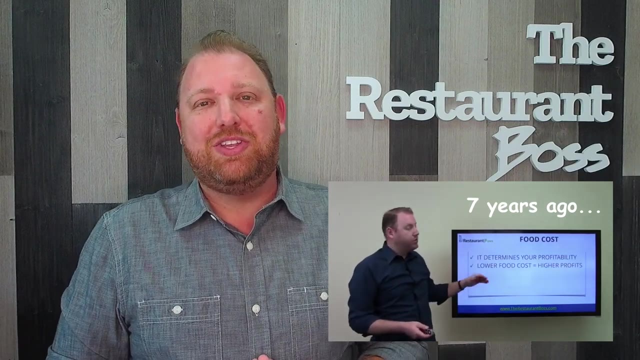 And most viewed videos. It's all about food costs: Everything you've ever wanted to know about food costs, The formulas used to calculate it, The questions I get asked the most about food costs And some of my simple ways to calculate food costs in your restaurant. 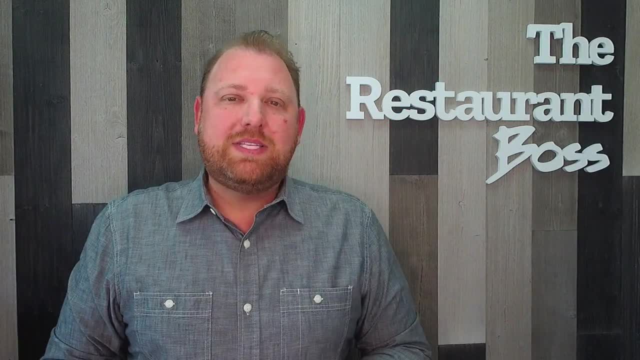 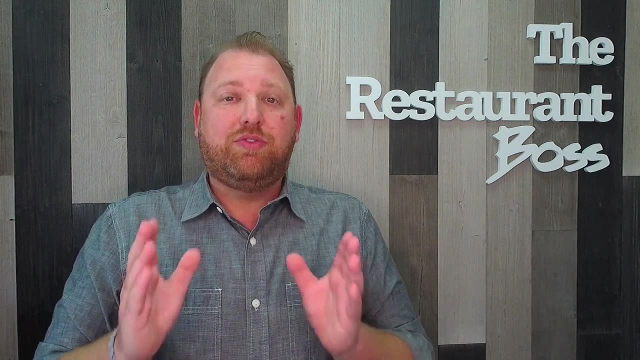 Coming up right now, But before we do that, I want to take a moment and thank my sponsor for this video: Radiant Digital Signage. You know, without all of you viewers watching these videos, commenting, liking, subscribing and sharing. 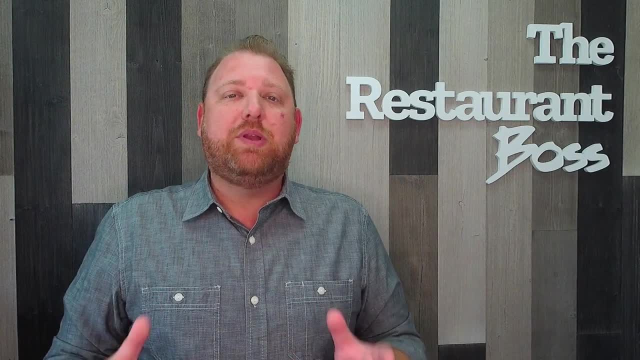 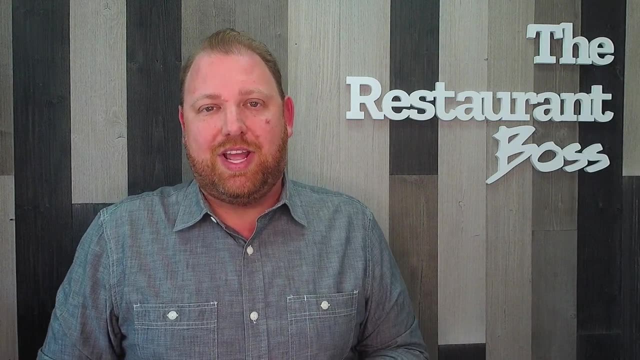 as well as the support of sponsors like Radiant, I wouldn't be able to keep bringing you these amazing videos free of charge, So I really want to thank Radiant for bringing us this video today. We've been in partnership with Radiant Digital Signage for over a year now. 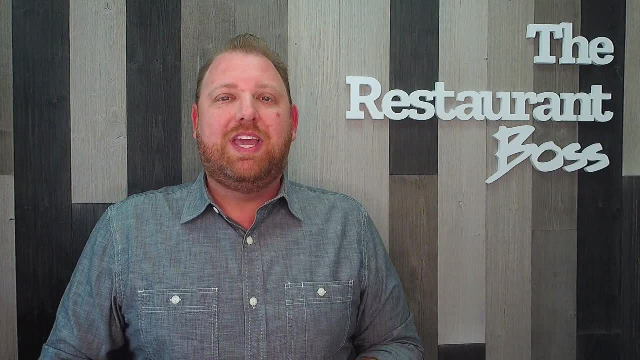 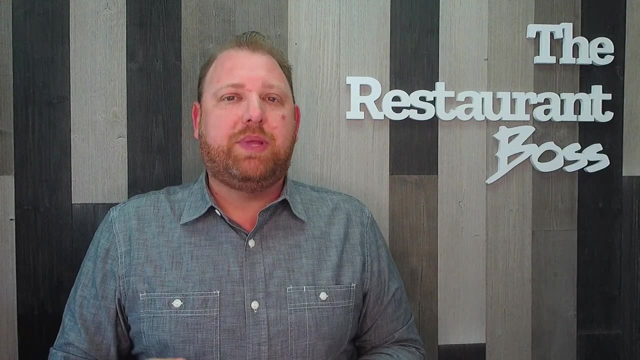 And, in my opinion, they are the absolute best in the business. if you're looking for a simple do-it-yourself solution, There are other options out there that are very expensive and very complicated, And you need a designer to set up your menu and your signage. 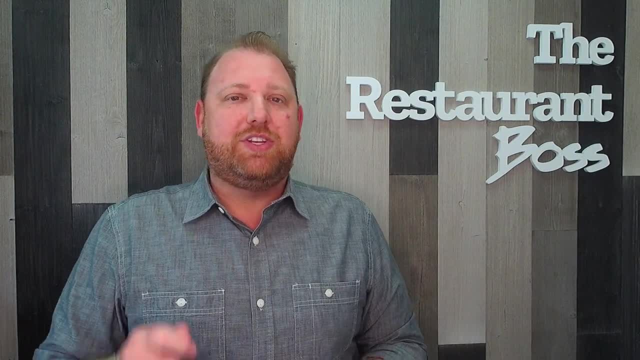 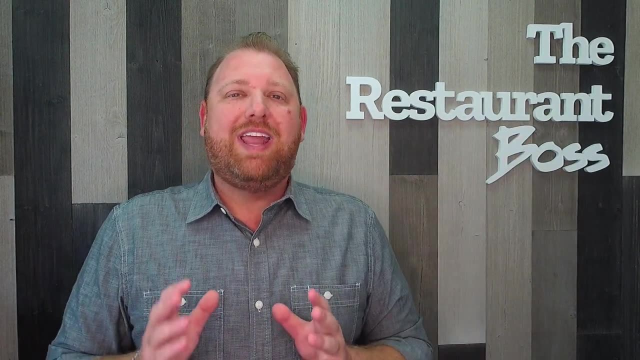 But with Radiant you can set up your menu, your signage, your advertising, You could put YouTube videos, social media, weather, any promotions you want on any television in your restaurant. Super simple, super effectively and it's super easy. 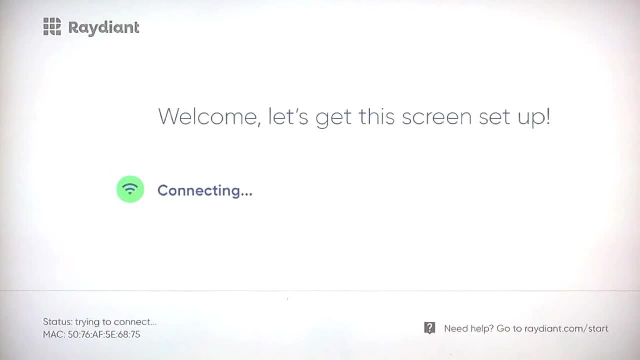 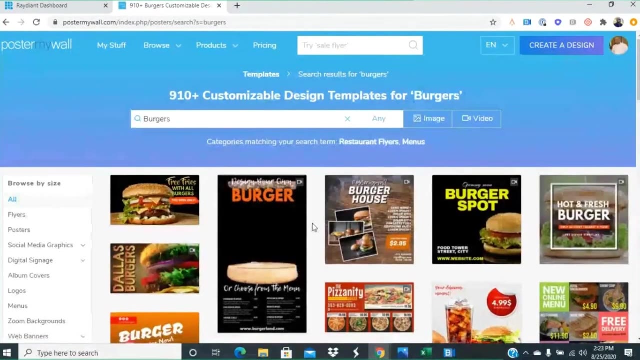 All you need is this little guy right here which plugs into the back of any TV, and a subscription through Radiant which includes access to a massive library of templates So you can create a menu or whatever you want in just a few minutes. 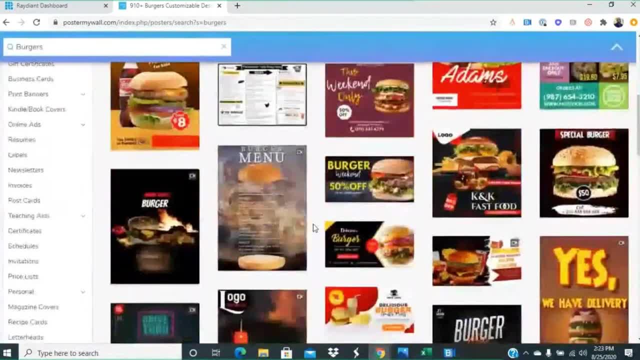 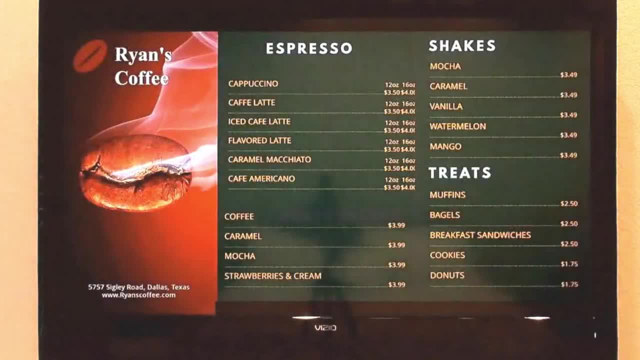 In fact, if you visit our website using the link in the card right up there, you can watch a video of us setting up a digital menu in about 10 minutes, from opening the box to pushing the menu live to a TV. And now Radiant has an integration with Toast. 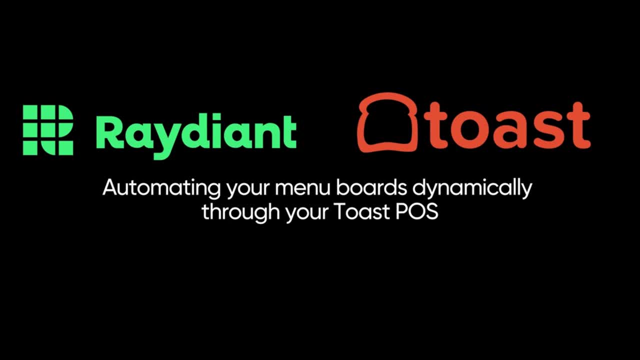 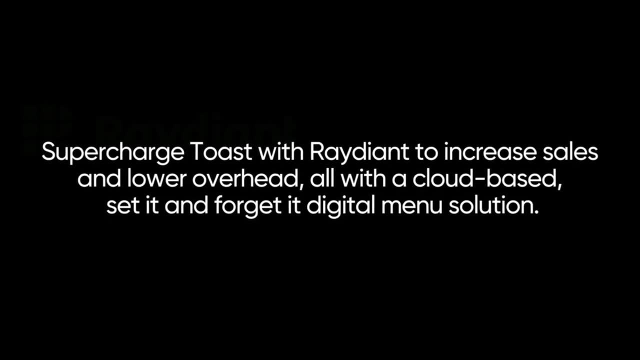 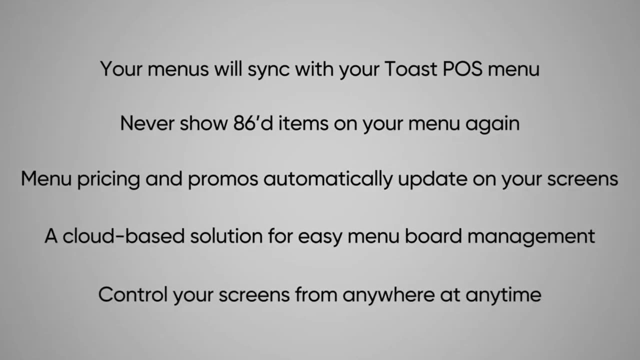 So for all of you Toast POS users out there, you can automatically import your menu into Radiant and then style it any way you want. Plus, if you run out of an item, it gets taken off of your digital menus automatically For more information or to set up a demo with a product specialist at Radiant. 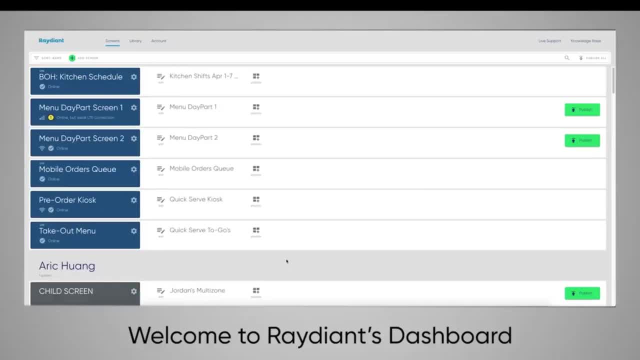 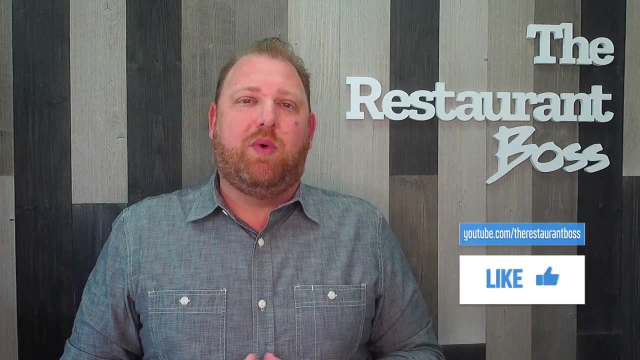 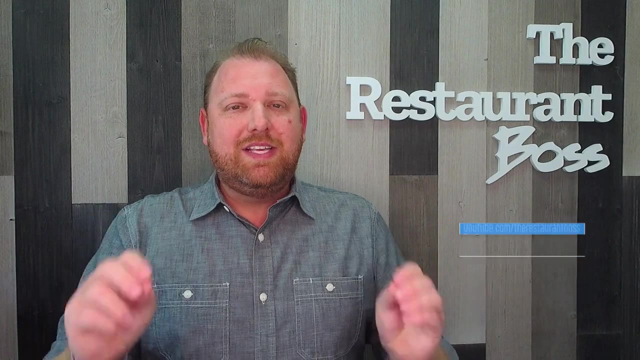 or to receive the special restaurant boss pricing with Radiant, please click on the link below this video. So the first major point I want to bring up when we're talking about food cost is the difference between food cost and plate cost. This gets confused a lot. 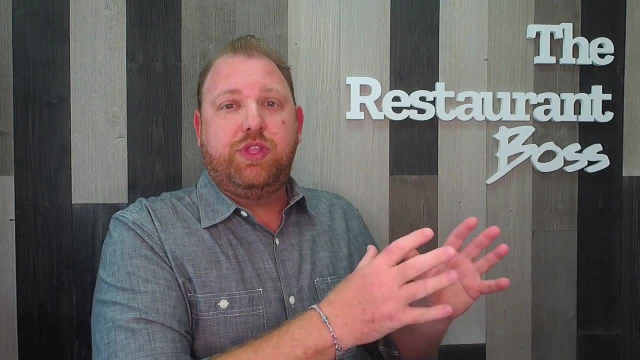 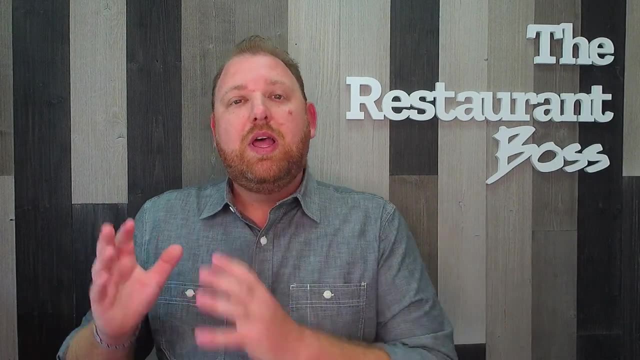 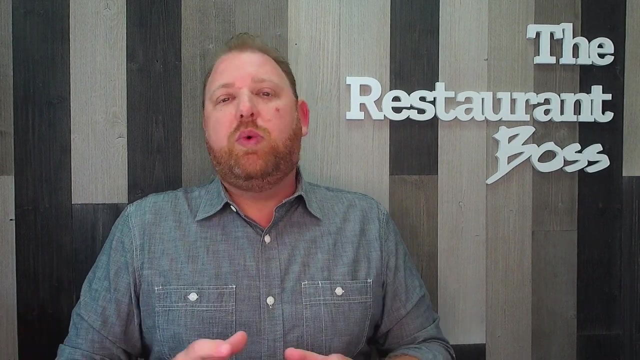 Food cost is the cost of the food that you use or that you purchase in a specific period of time across your entire restaurant. Plate cost is just the cost to produce one specific plate. So please, when you're emailing me questions or commenting below or just having conversations about food cost in general, 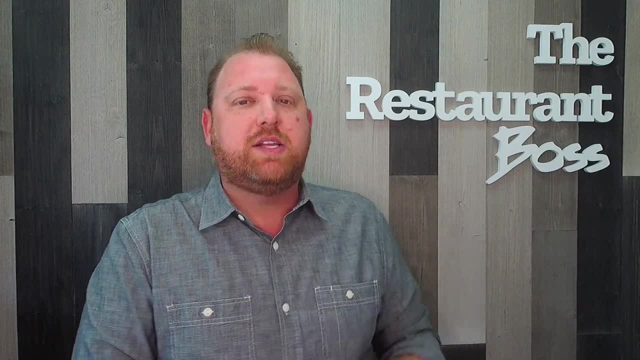 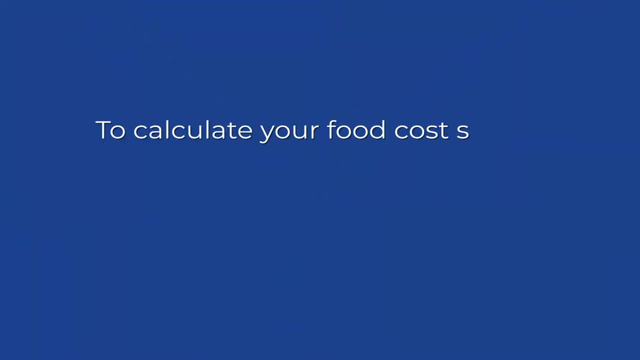 make sure to use the correct verbiage- the difference between food cost and plate cost- Because this can get a little confusing as we move forward here. To calculate your food cost, simply divide the amount you spend on food in a period by the amount of food sold in that same period. 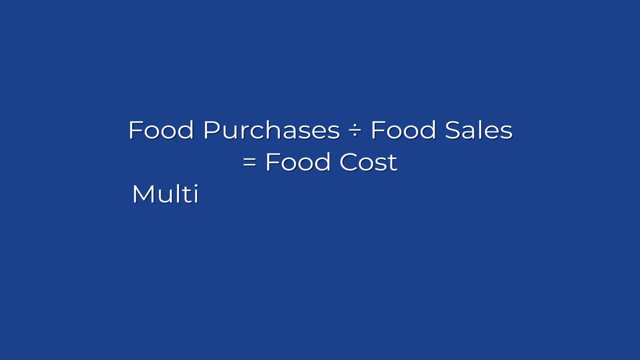 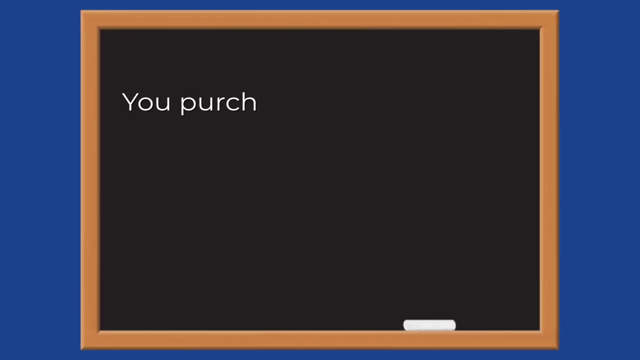 So here's the formula: Purchases divided by sales equals food cost. Then just multiply that food cost by 100 to get a percentage. So as an example, let's say you purchased $2,500 in food this week and sold 10,000 in food. 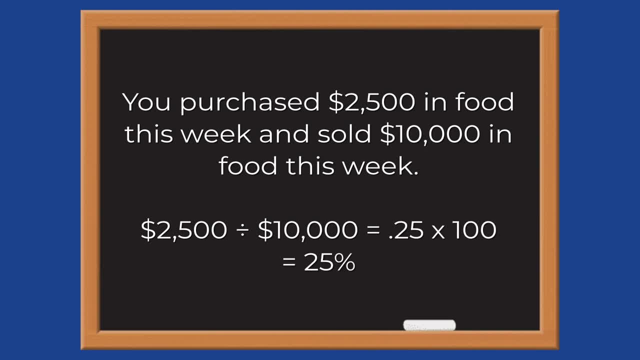 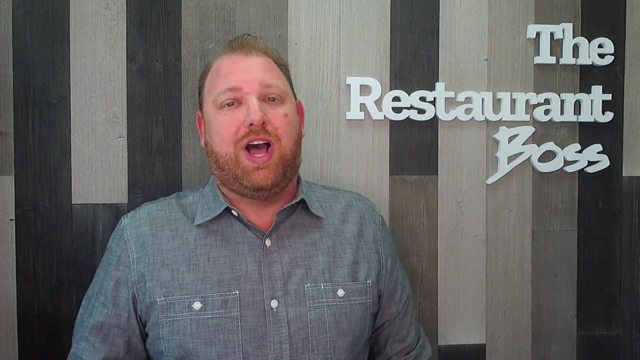 Then 2,500 divided by 10,000 equals 0.25.. Multiply that by 100 and you get your 25% food cost. Some of you are going to want to use inventory to create a more accurate food cost. We're going to talk about the pluses and minuses of this later in the video. 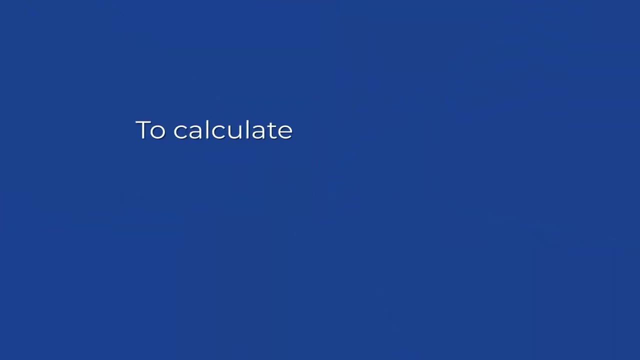 But for now, let me share that formula with you. To calculate food cost using inventory, we first need to figure out our usage. To figure out usage, we need to take beginning inventory plus purchases and then subtract ending inventory, which will give you usage. 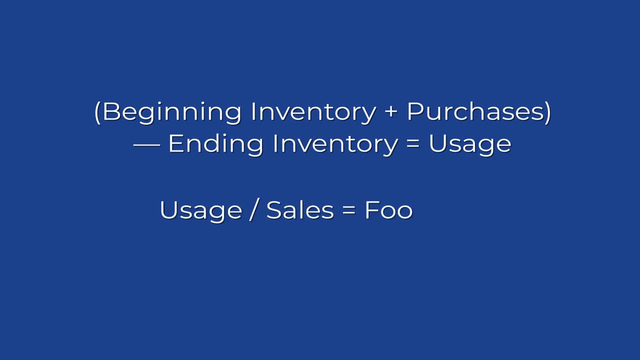 So then we take our usage and divide that by sales, which equals your food cost, And again just multiply by 100 to get your percentage. So as an example here, say you started a week with $1,000 in food on your shelves. 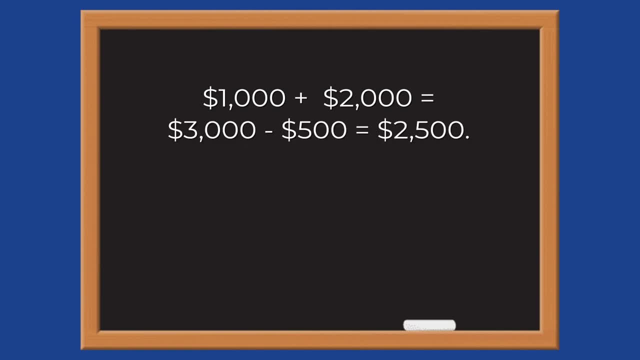 You purchased 2,000 and then ended the week with 500 of food left on your shelves. That would be 1,000 plus the 2,000 you purchased, which is $3,000.. That's 3,000 in food available. 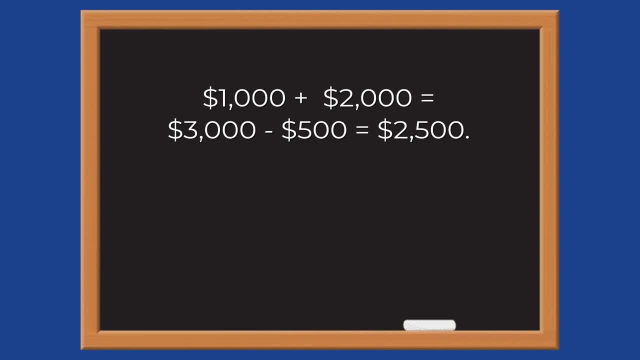 But then at the end of the week you have 500 in inventory. So now you're left with 2,500.. Now again, as in the previous example, if we take that 2,500 divided by your 10,000 in food sales, 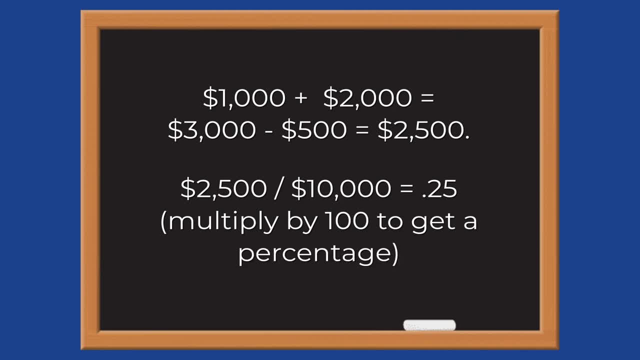 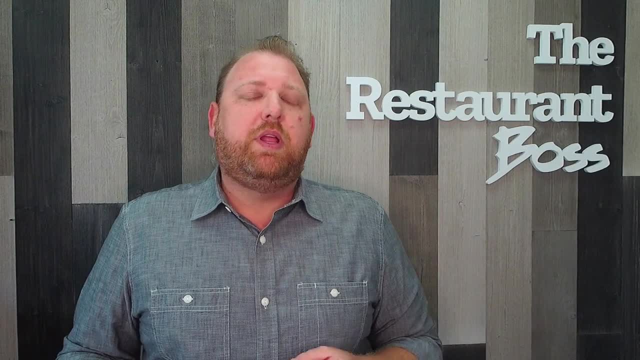 for this particular week, you're going to get 0.25.. Multiply that by 100 and you get your 25% food cost. Now the same formula applies to plate cost. Let's just use smaller numbers. Let's say that you're costing out a burger on your menu. 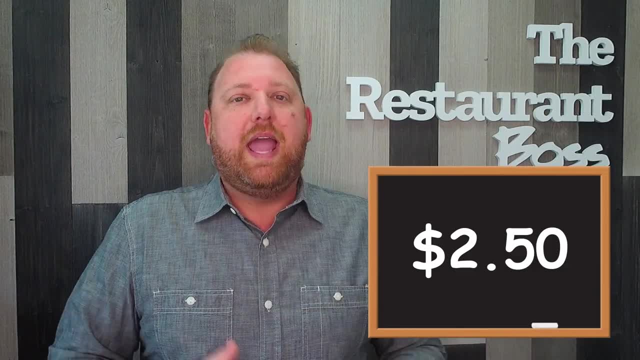 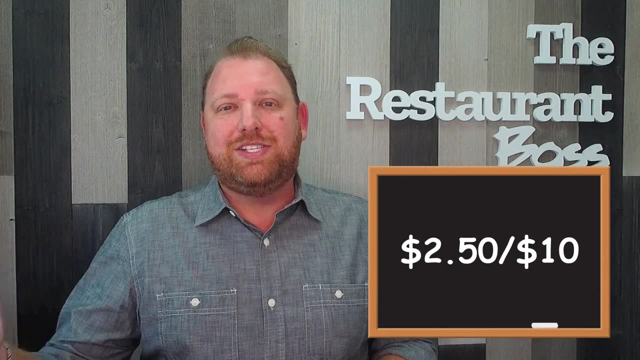 The burger costs you $2.50 to make it and you sell it for $10. Well then, we just simply divide the $2.50 divided by the $10 that you sell it for, and you're going to get the same 0.25 times 100, which is 25%. 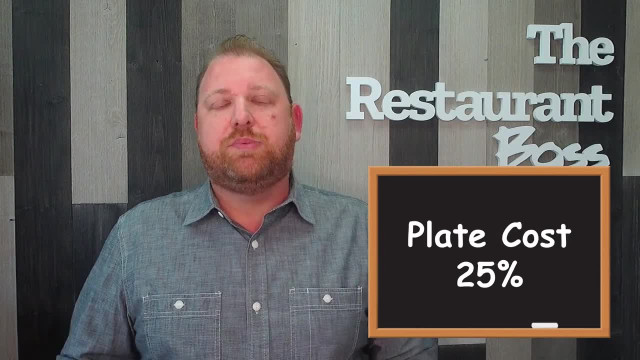 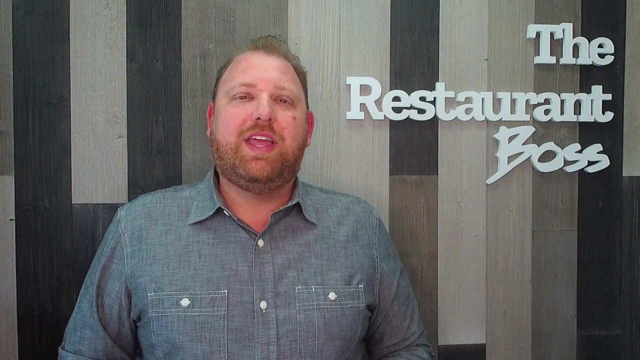 So in this case, your burger cost, the plate cost to produce your burger- is also 25%. So the question I get the most is, Ryan, is there an inventory system that you recommend? I want to get a very accurate food cost in my restaurant. 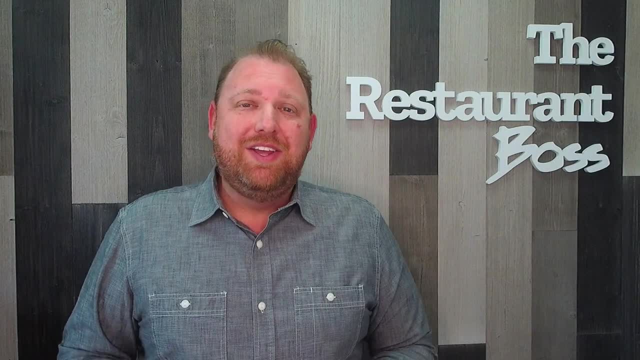 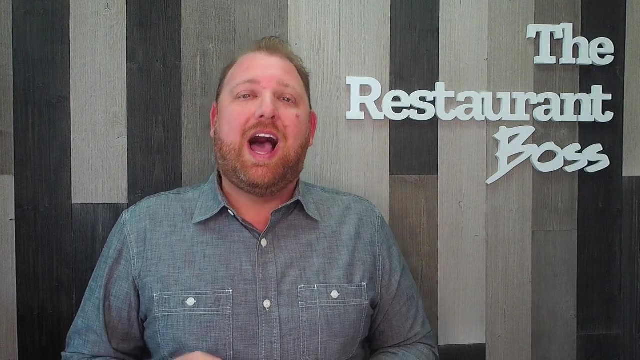 The answer is no. I personally hate restaurant inventory and unless your restaurant is doing approximately $5 million out of its location, I do not suggest that you take the time, the energy, the effort and the money that it's going to take you. 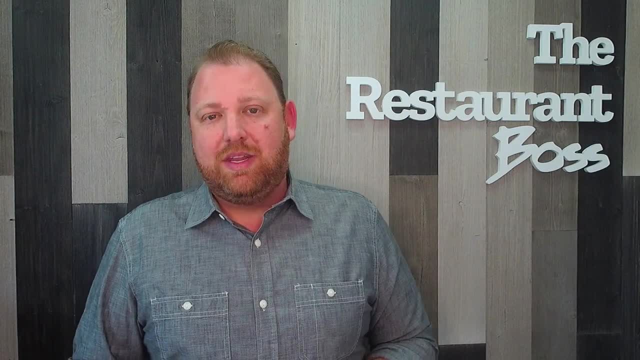 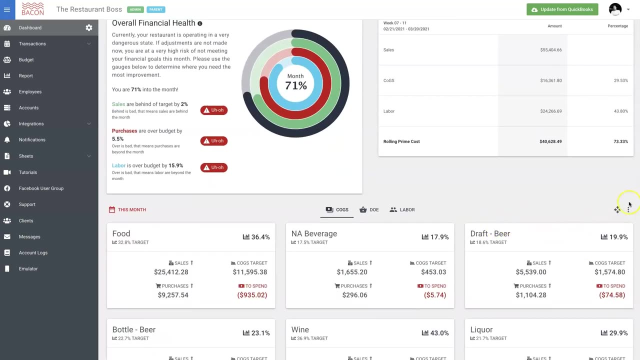 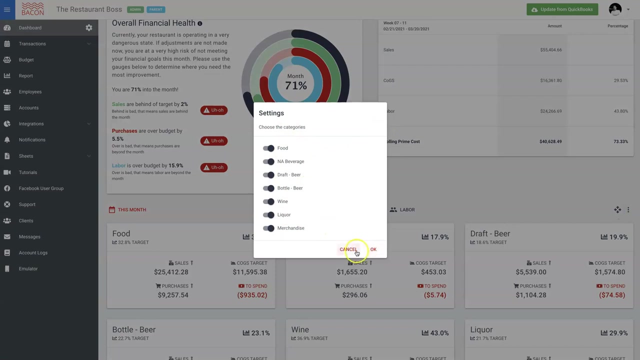 to get an accurate food cost using the inventory method, which is why we created a software tool called ClickBacon. Now ClickBacon will allow you to get a very accurate weekly, monthly, rolling, quarterly, yearly food cost, labor cost, beer cost, wine cost, total cost. 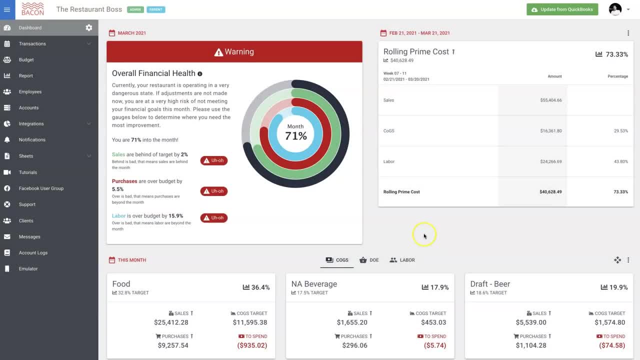 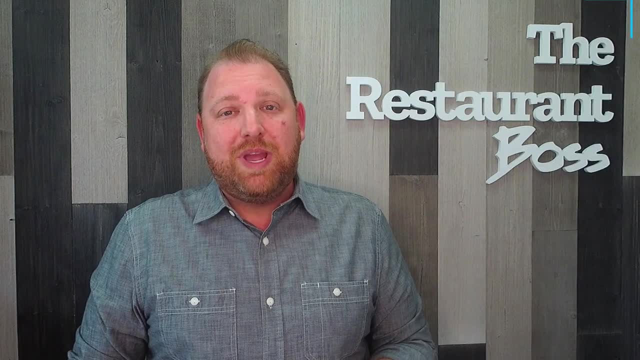 cost of goods sold, direct operating expense, prime cost, whatever it is that you want in your restaurant without having to take inventory. For more information on why I hate inventory so much, go ahead and click that link above. I've got a whole video about that. 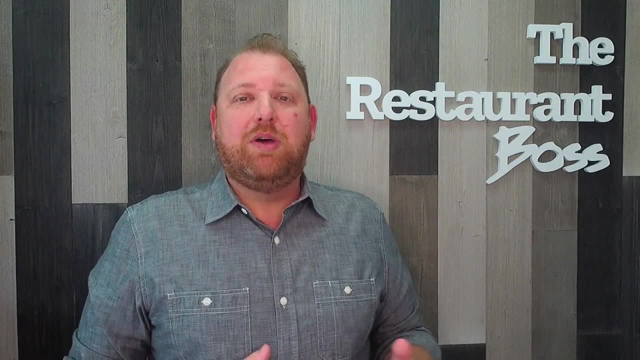 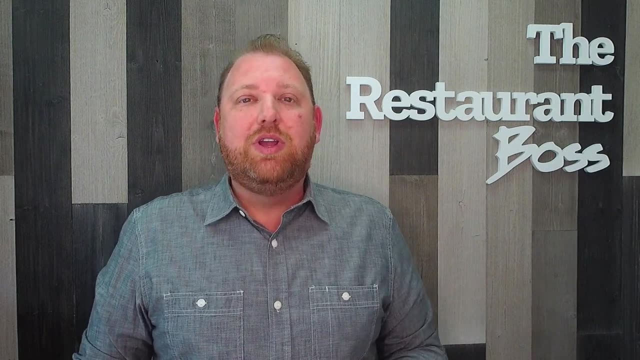 Another thing that people ask me is, Ryan, how come ClickBacon doesn't do this? or do you have a software tool or a spreadsheet that you recommend for costing out particular recipes, for getting plate costs? And again, my answer is no. 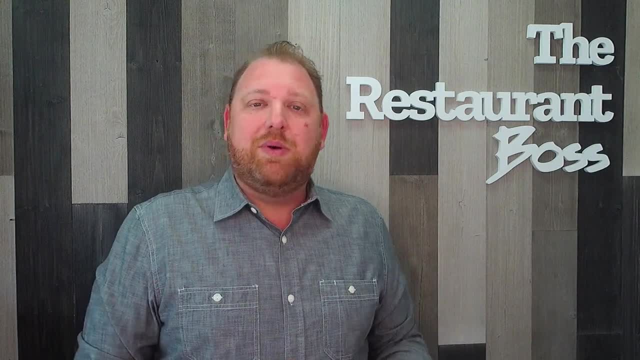 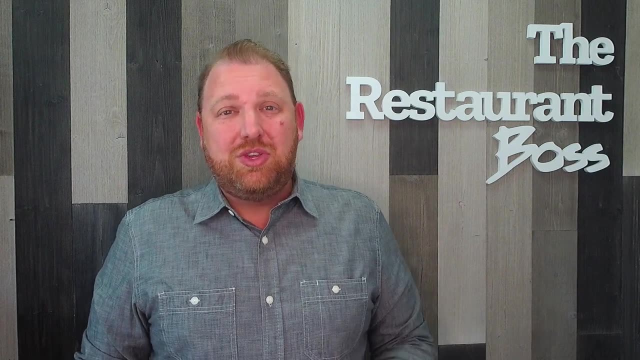 And I know a lot of people out there are going to think this is crazy, but when I was operating restaurants and even still to this day working with clients, when we're trying to figure out the plate cost, we basically just use a scratch piece of paper. 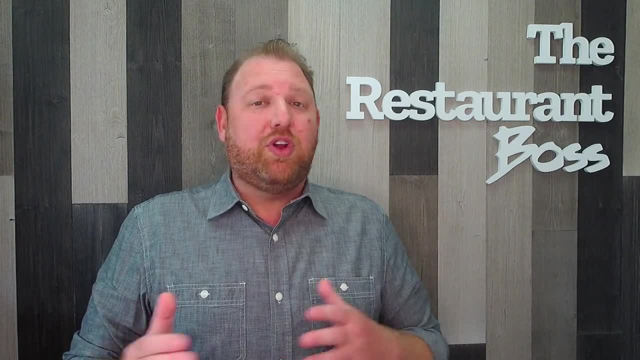 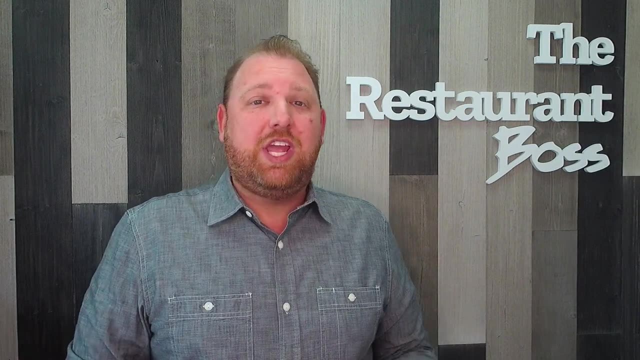 because the reality is, even if you're accurate or if you're off by a couple of pennies, that's not going to change the price you're going to charge for this item to your guest. You're not going to change your hamburger price from $10.35 to $10.45.. 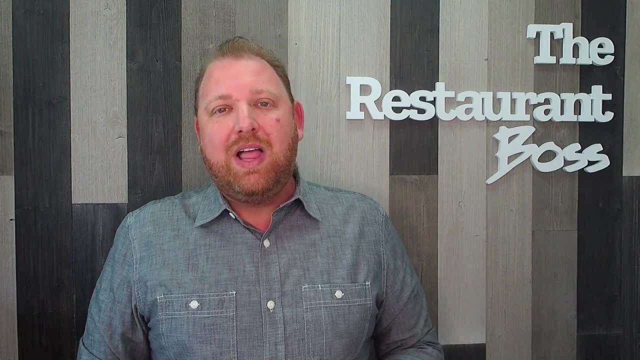 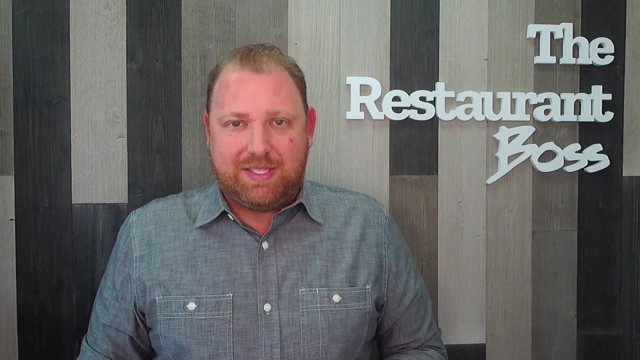 Because it costs you two cents more to make it, When, in reality, what you're going to do, or what you should do- and in that video we're going to explain it- is you should price your products at where the market demands. Now, we also are only interested in your full menu. 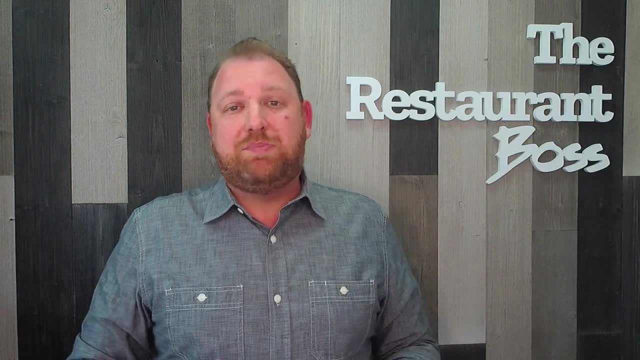 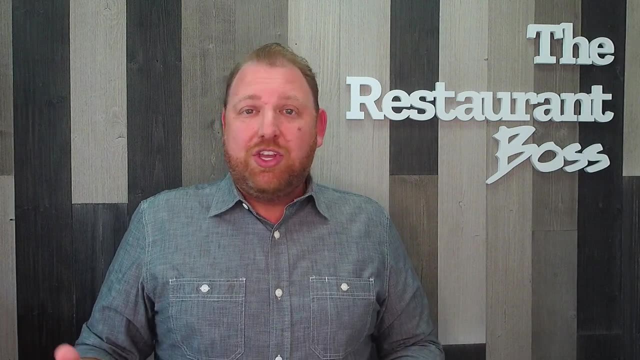 because you may sell french fries at a 15% food cost but then a cheeseburger with bacon and avocado might be at a 50% food cost, because at a 25% food cost your guests aren't going to pay the $17 or $18 that you would need to charge. 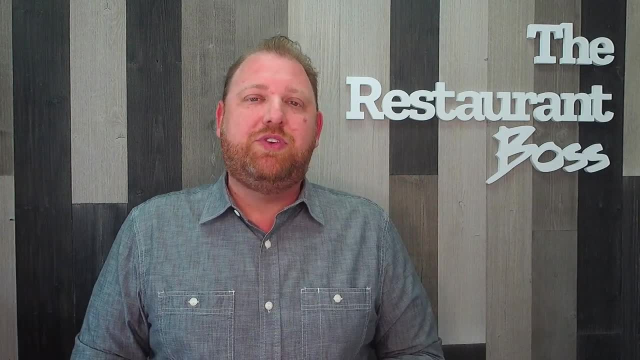 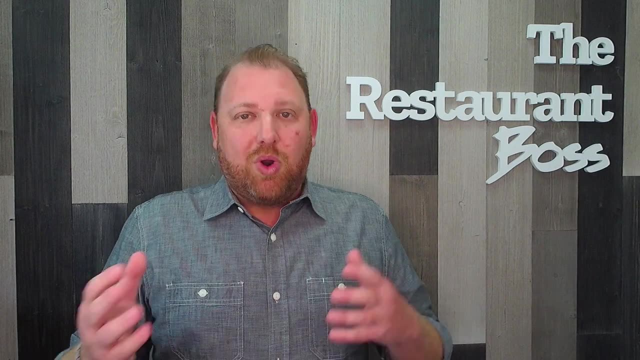 for that burger, But because it's more expensive. at a 50% food cost, you're still making enough money. Again, I don't want to get into too much detail in today's video. I just wanted to go over some of the more common questions. 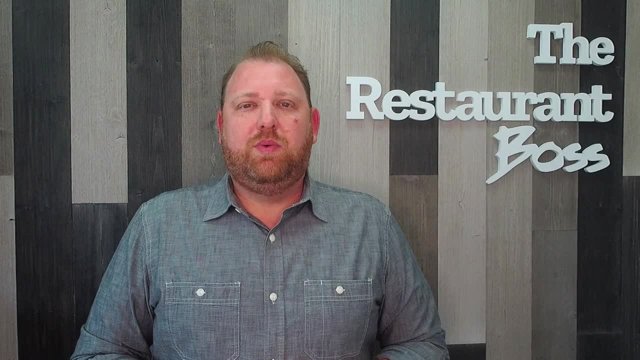 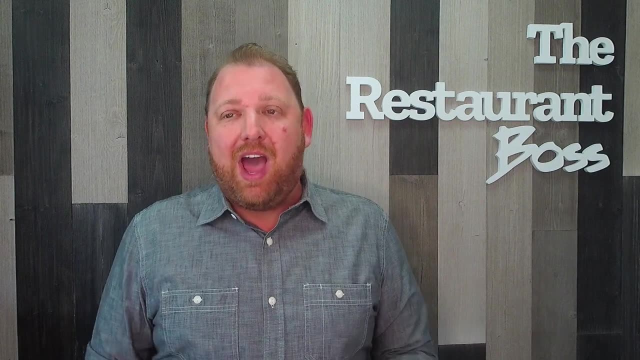 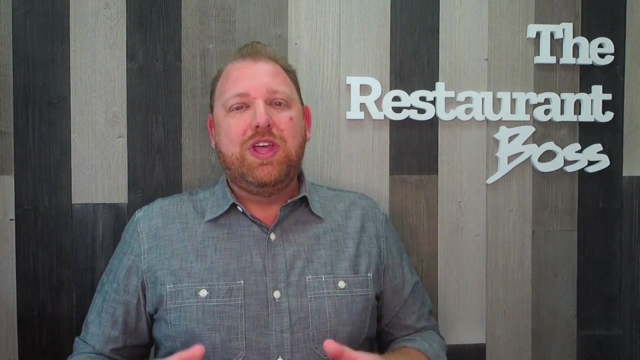 and topics that are brought up regarding food cost. While this topic of food cost is incredibly important and incredibly in-depth- I could literally spend hours talking about food cost- I really just wanted to recreate this video from over seven years ago that gives you the overview- my most important thoughts on food cost. 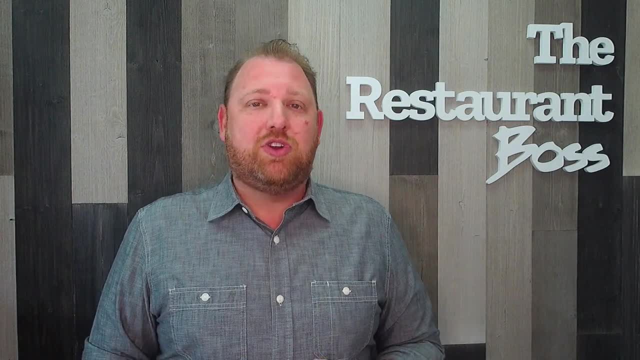 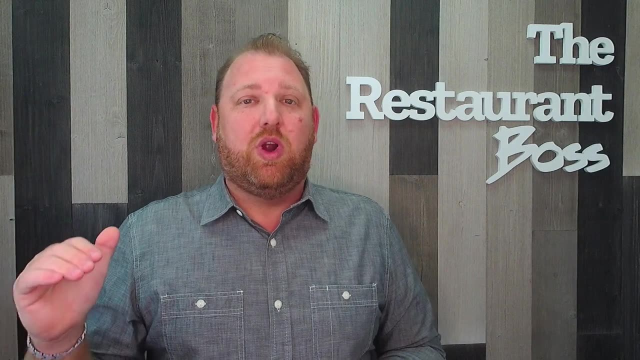 If you're interested in learning more about food cost, come to TheRestaurantBosscom, go to our free videos or our video blog. click in the search box or in the category for food- food cost, cost savings, that we have different categories in there. 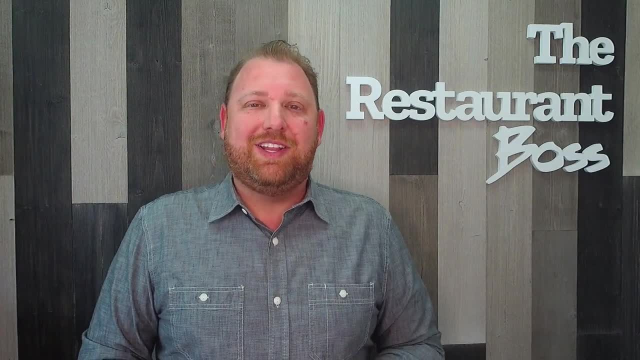 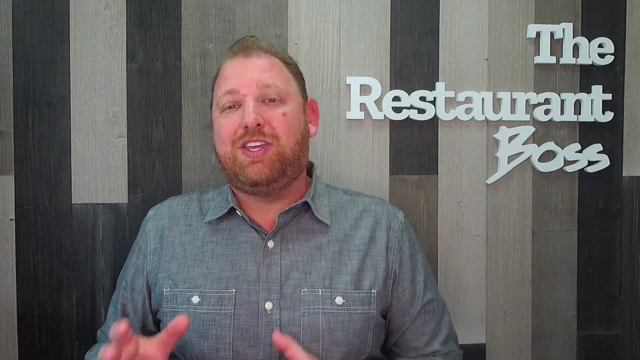 and you're going to find a ton of videos related to this topic And, trust me, I'm very opinionated on what I think you should be spending your time on and what I think you shouldn't. Well, food cost is very important. 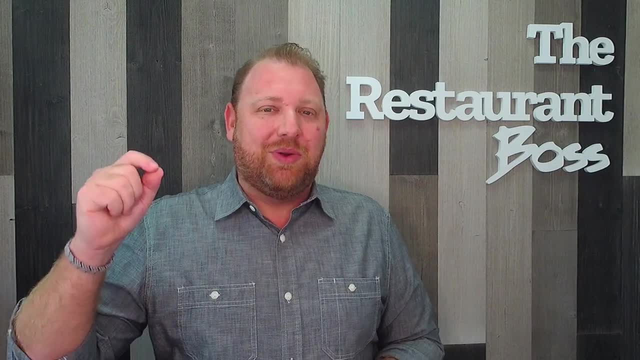 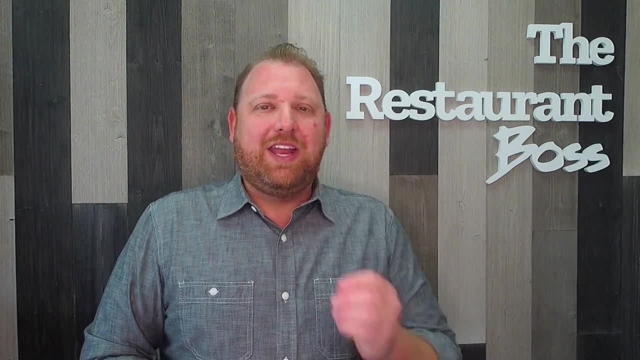 and I know a lot of you out there are going to say that this is terrible, that, Ryan, you have to be taking inventory in a restaurant. What are you talking about? I have different thoughts on it. I know how busy you are as a restaurant operator. 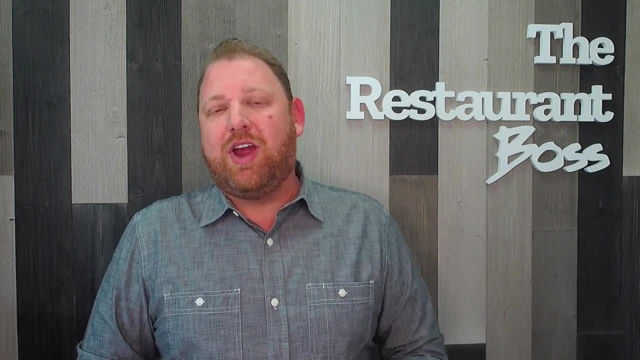 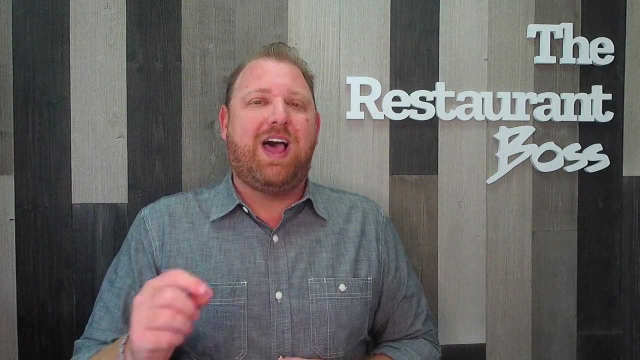 and I think you should be spending your time worrying more about hiring a great staff, training them, making sure you're exceeding your guest expectations and getting your food cost. don't get me wrong: it's important, but not down to the penny. 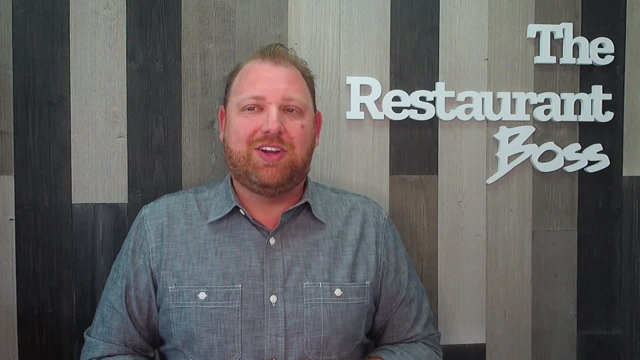 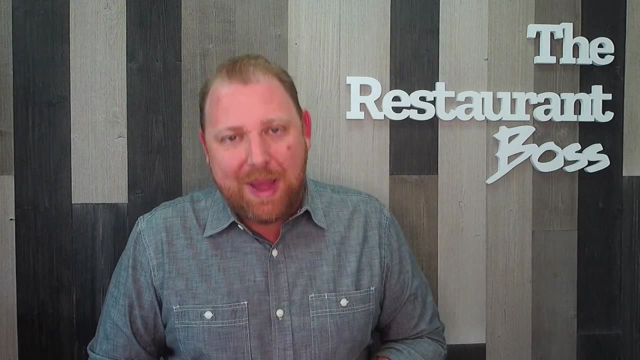 not unless you're up in that four, five million dollar a year range. You just shouldn't be spending too much time on that. I hope you enjoyed today's video and remember: systems create freedom, freedom creates value and value creates scale. 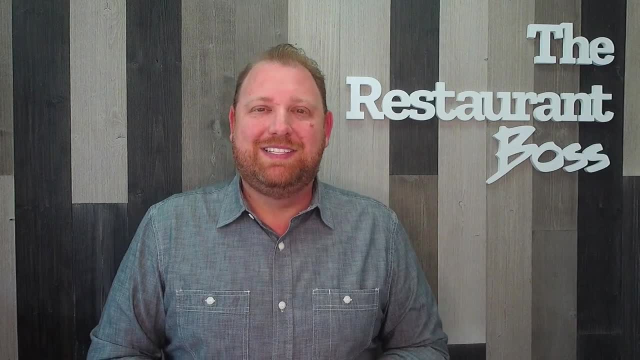 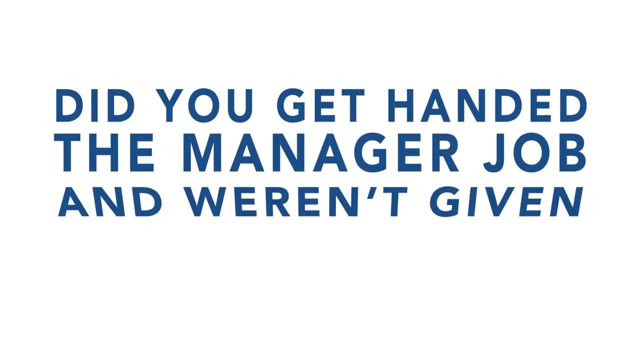 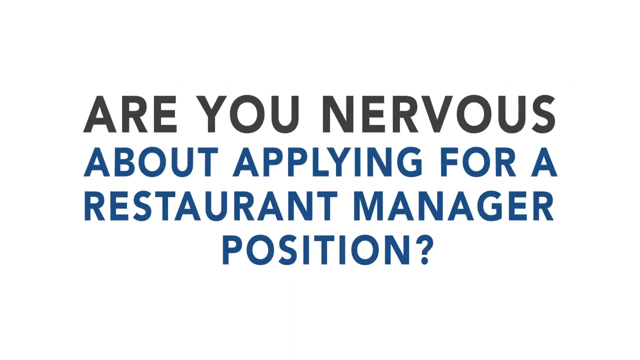 Have an absolutely amazing day Bye-bye. Want to improve your skills as a manager and make more money? Did you get handed the manager job and weren't given the support you need? Be generous about applying for a restaurant manager position. Managing restaurants, bars and kitchens is not easy. 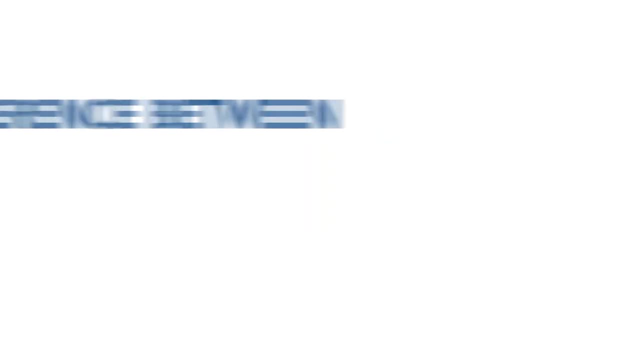 I know I have been there. I want to help. The difference between where you are now and where you want to be is a plan and some new tools. That is why I created the Restaurant Manager Certification. It's a boot camp for aspiring restaurant leaders.